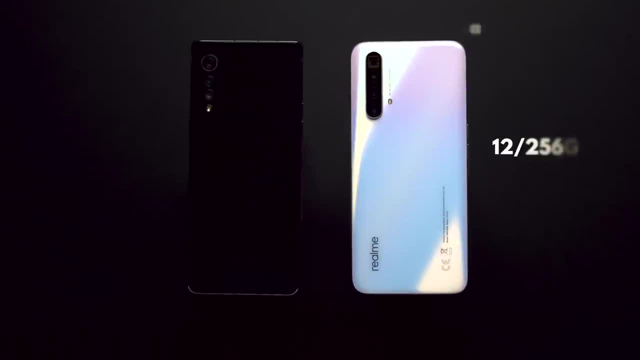 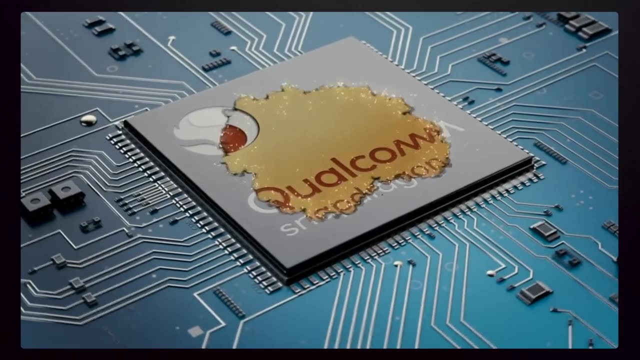 but instead comes with a periscope camera. The X3 has more and a faster memory, and the two phones don't even share a processor. Of course, neither could afford the flagship Snapdragon 865, because Qualcomm went crazy with the pricing this year. But 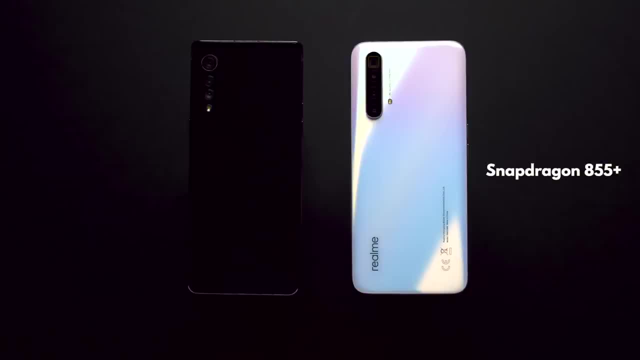 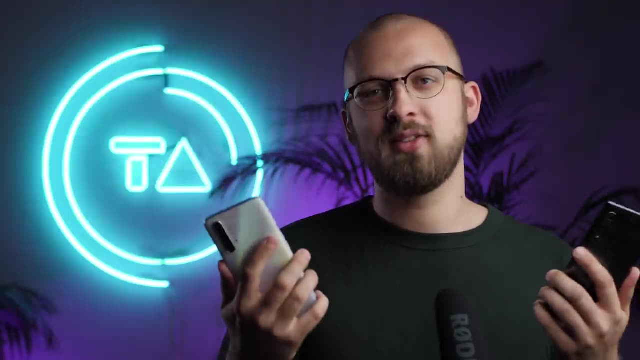 interestingly, Realme chose to go with last year's 855 Plus, while the LG chose this year's 765.. There's almost no overlap between these two devices, and what drives these massive differences is something that you, as a consumer, very rarely think about. 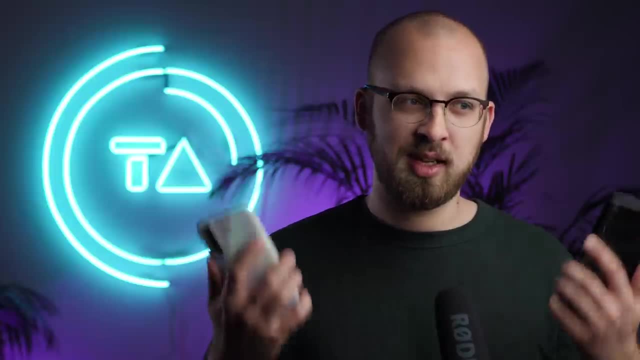 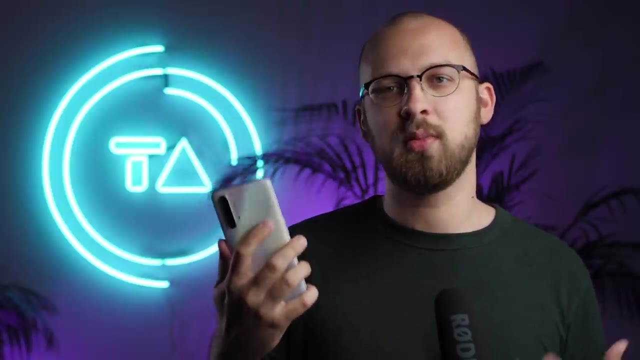 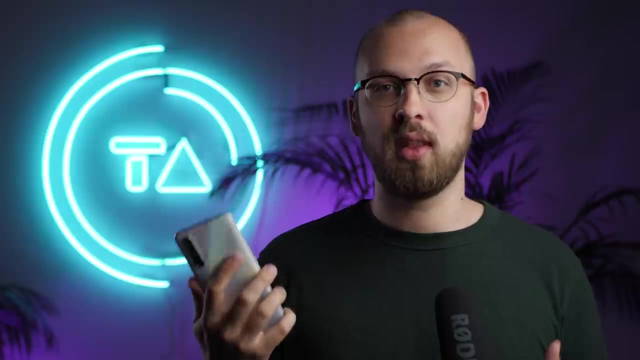 but something that successful companies completely obsess over. It's their prospective selling processes. Let me explain. Okay, let's start with Realme first. How does the typical Realme customer find, research and finally purchase a Realme phone? Well, we know that Realme sells phones almost exclusively online and we know that their 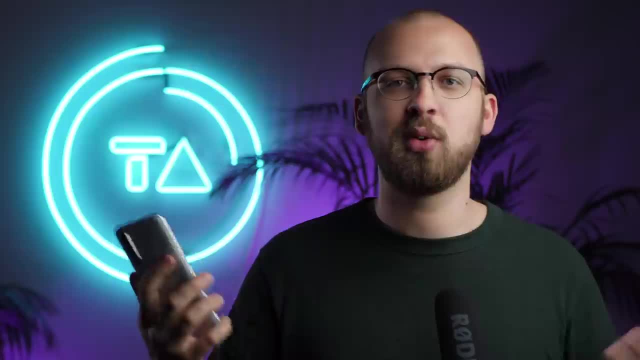 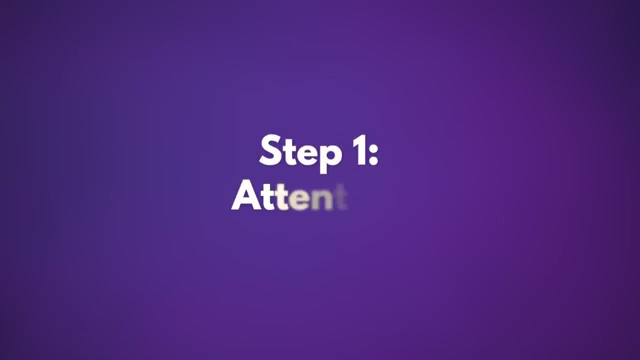 target audience consists almost exclusively of spec-hungry tech enthusiasts, so we actually know what their purchasing process looks like, and it consists of three main steps. First, Realme needs attention. How does one grab the attention of a tech enthusiast online? 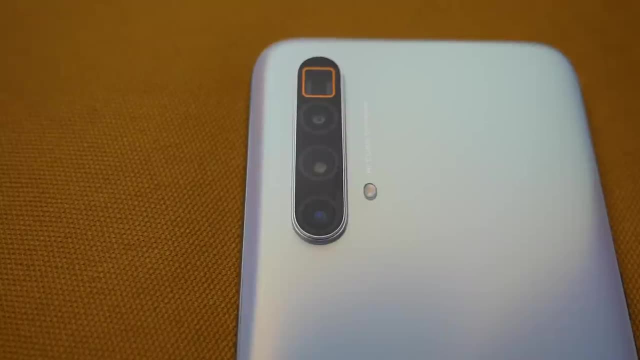 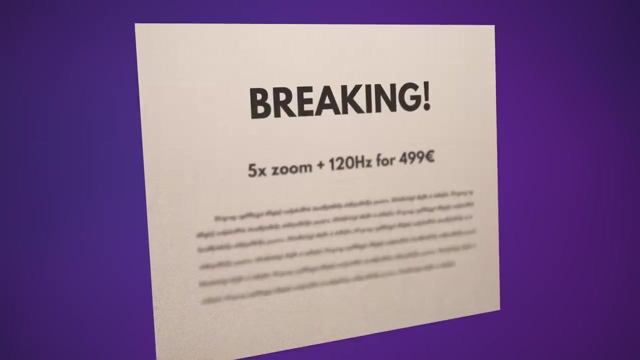 Well, putting wild features like a super zoom periscope camera and the 120Hz screen into a phone that costs half as much as the competition will sure do the trick. Those features easily generate headlines that those people who closely followed the latest tech trends are bound to pay. 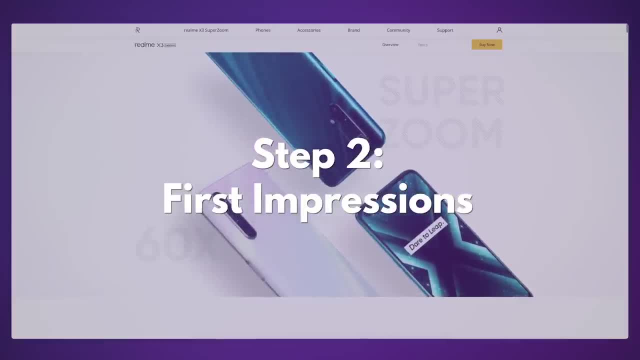 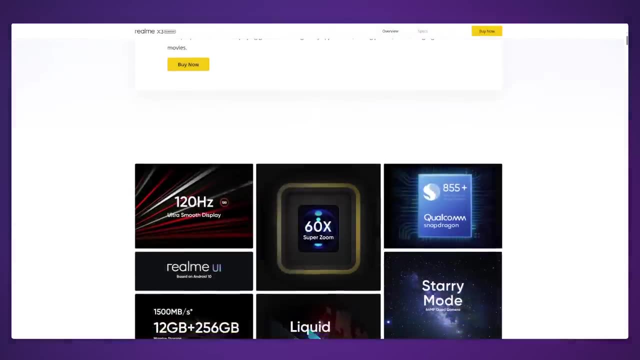 attention to Second Realme needs to nail the first impressions. The first thing a tech enthusiast checks in a phone are the specs. of course We can't touch or try a phone ourselves online, so we use numbers to decide if a phone is even worth our time and Realme. 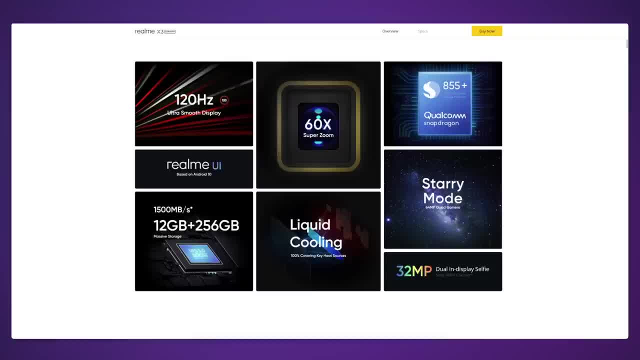 knows that. So the processor, the amount and speed of memory, the battery size, the charging speed, the number and resolution of cameras, basically anything you can attach a number to, they made sure it looks solid. So on to step three, then, where the customer 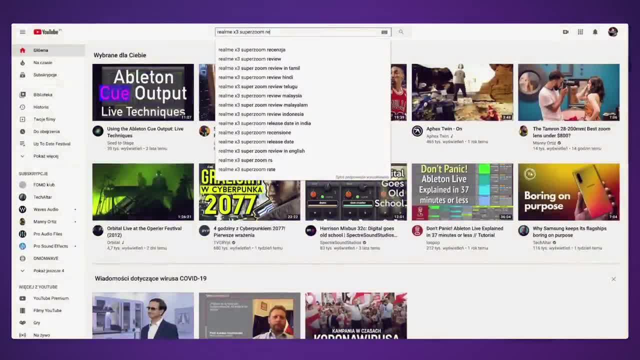 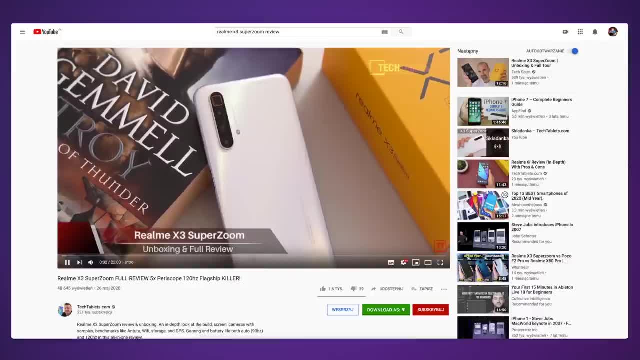 goes on to make more in-depth research, usually through watching online reviews, best of all on YouTube, so they can actually see the phone in action, And Realme has made sure that their phones make a positive impression here as well. The X3 looks solid on camera. It has features. 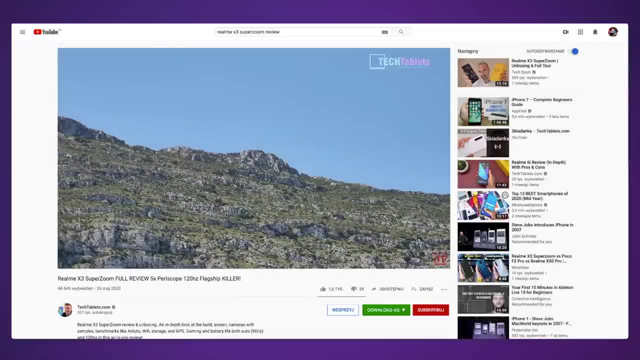 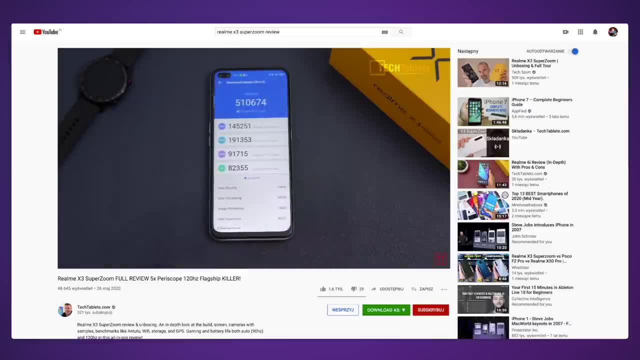 scope camera which can easily be demonstrated visually, and they make sure that all the things reviewers can easily objectively measure, like performance benchmarks, battery charging tests and whatnot, they all look positive. In other words, this phone is optimized to look great on. 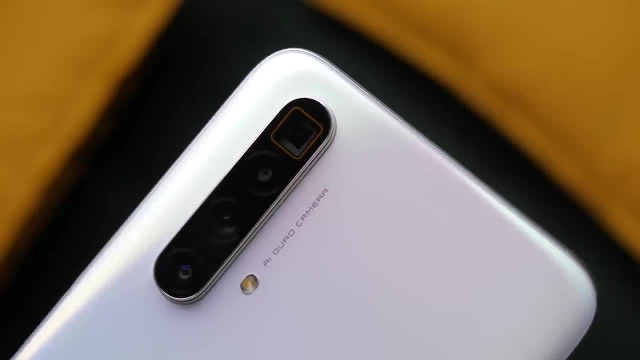 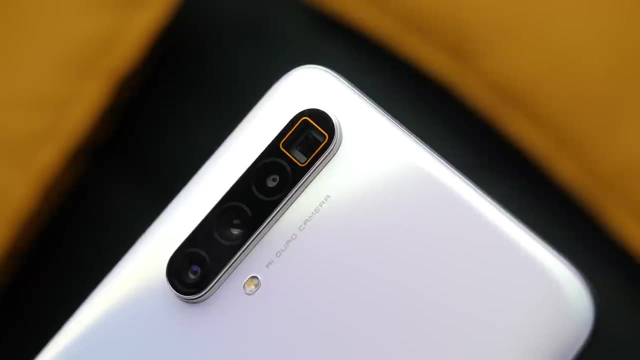 all online touchpoints, Realme's website, spec sheets and online reviews as well. So tech enthusiasts going through this process see it positively and make a purchase. Where's the hook? Well, I have a question for you. You've been looking at this. 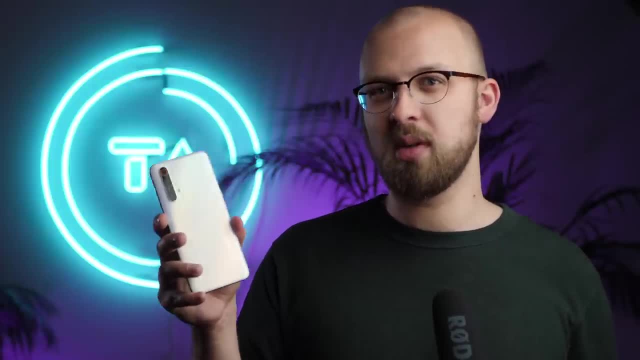 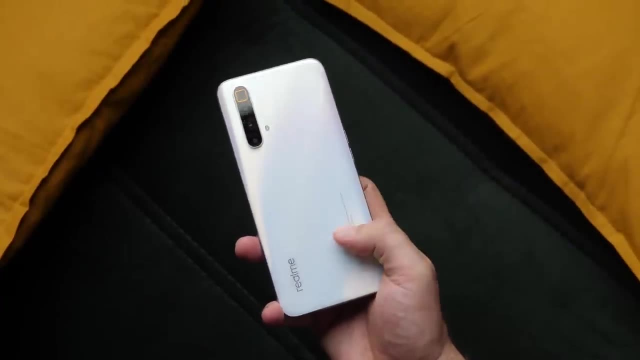 very phone for the last couple of minutes. What materials do you think Realme has used on the back and on the frame? I assume that most of you just assumed it's glass or metal, as did I when I first just saw it online, But no, the X3 Superzoom is made entirely of plastic. 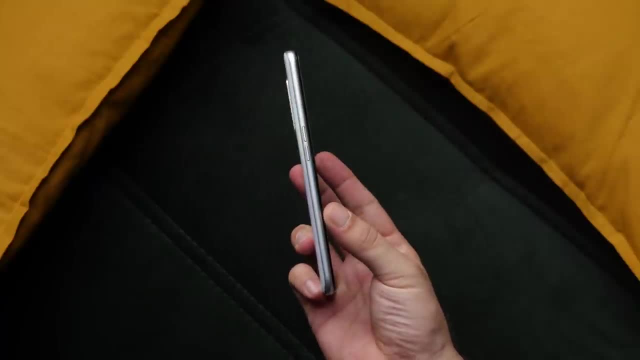 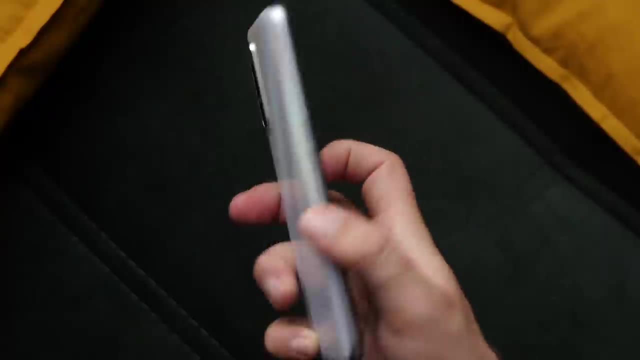 Pretty nice quality plastic actually, and I don't personally mind plastic at all. but this does highlight something pretty fundamental about Realme's purchase process: The customer never sees, hears or touches the device directly before the phone is placed on the back of the phone, And that's why it's so important to make sure. 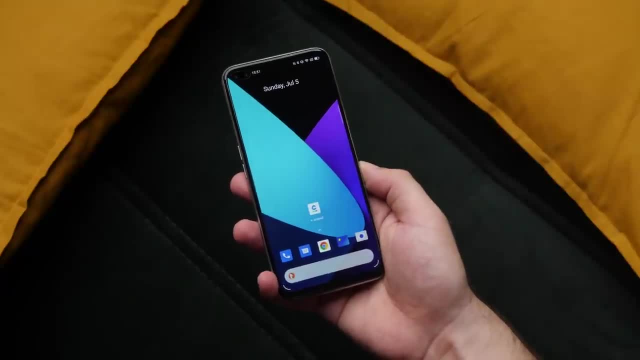 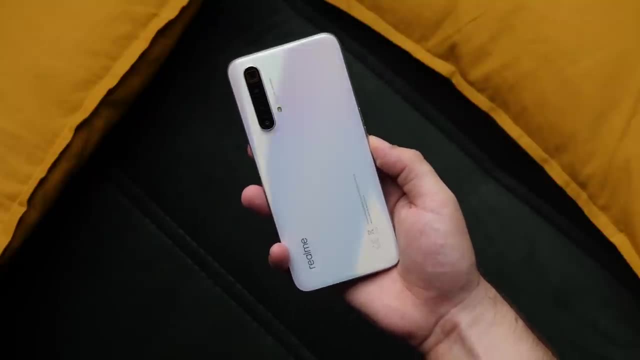 they buy it. And sure, good reviewers might try to convey their feelings to their viewers, but what a phone feels like in your own hands is simply impossible to accurately get from a video. It's not something that I can really show on camera. It wouldn't really show up on a spec. 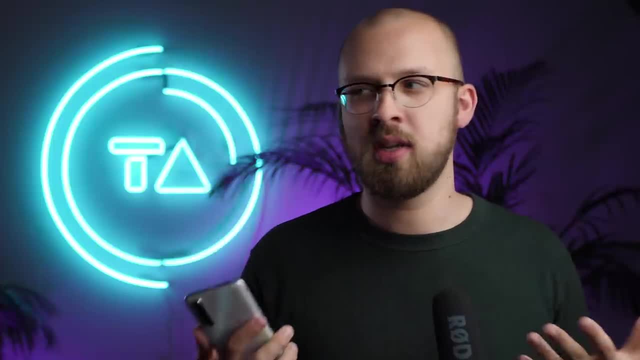 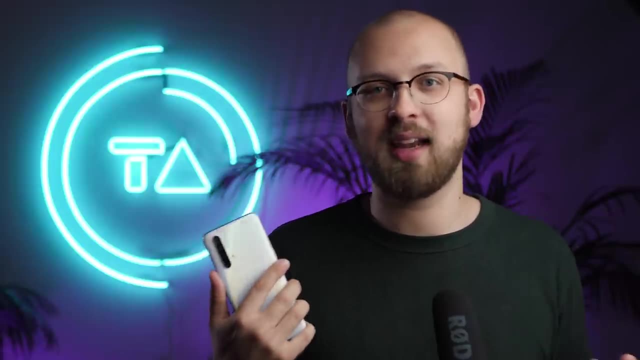 sheet either, because it's very difficult to quantify and measure And it just feels subjective. So reviewers tend to not want to talk about it too much, because our audiences don't like it when we become subjective and we just talk about our feelings instead of the. 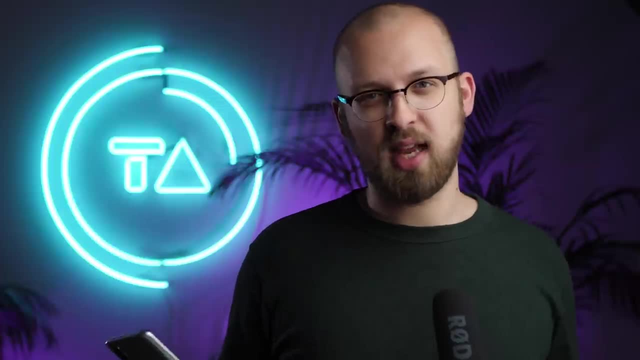 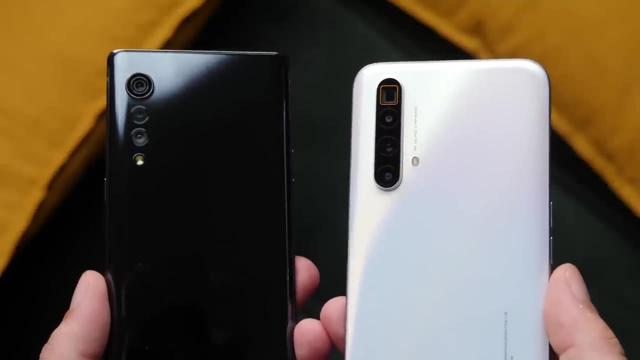 objective truth. So Realme just doesn't really optimize for that. The second you hold the X3 in your hands, it just feels significantly cheaper than, say, the Velvet Again. I've personally long advocated for function over form, but it's clear that the choice of 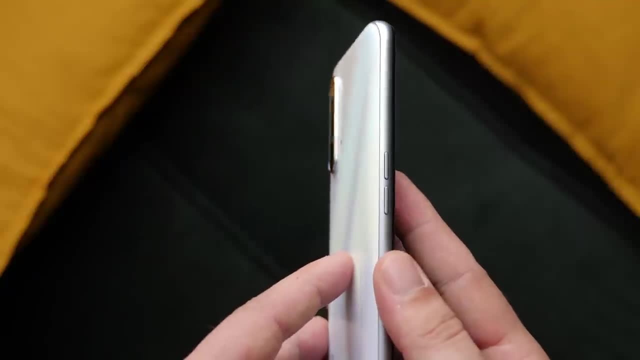 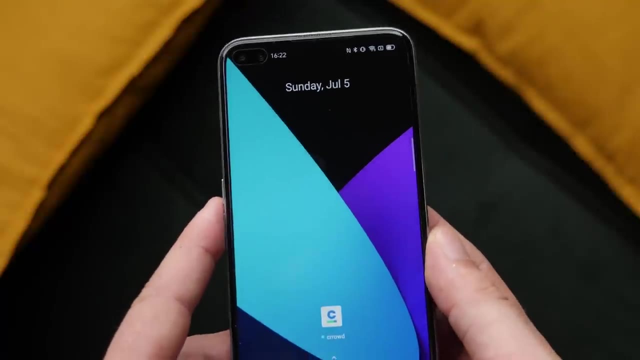 materials, the thickness, the weight, the way that single bottom firing speaker sounds, the way the buttons feel, the way the haptic engine vibrates, the colors and the brightness of the screen- all of the things that I myself vividly experience with my own. 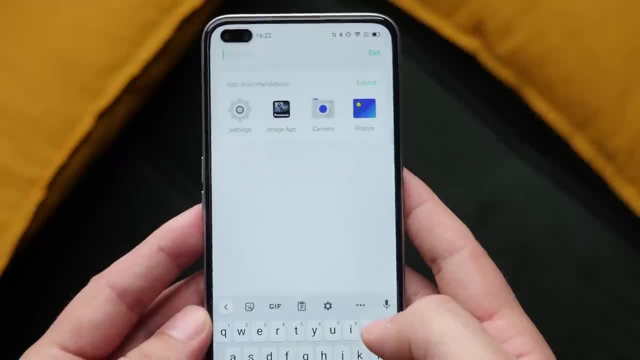 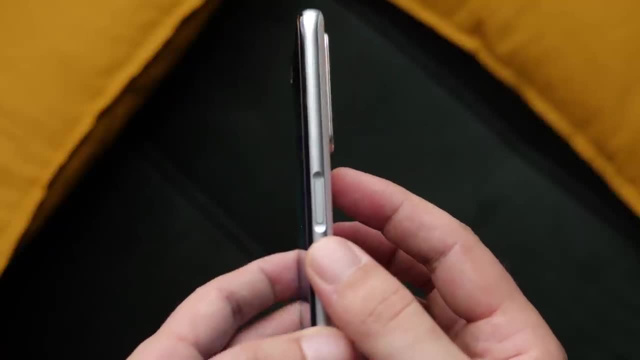 senses but that I can only vaguely describe to you. all of those just feel significantly cheaper than the LG And none of these experience things, for the lack of a better term are a deal breaker in my opinion. But it is clear that Realme had to cut some corners to be able to afford all. 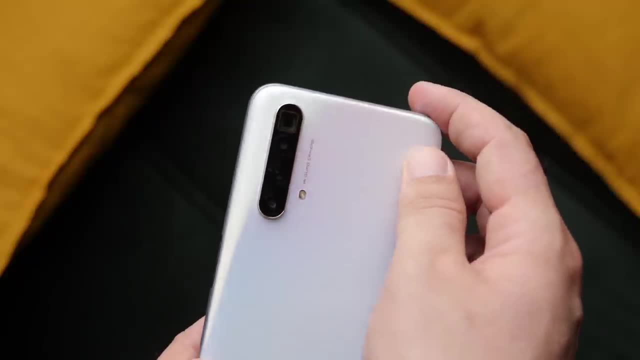 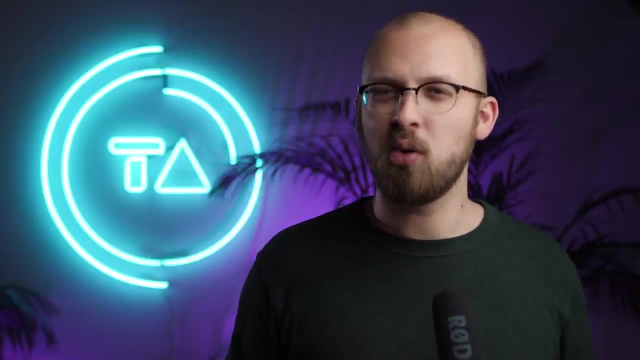 of those crazy specs and these were the corners they decided to cut Makes sense, after all. these are all things that the typical Realme customer and the typical Realme purchasing process would only really realize once they hold the phone in hand, And that, for Realme, means after the purchase. 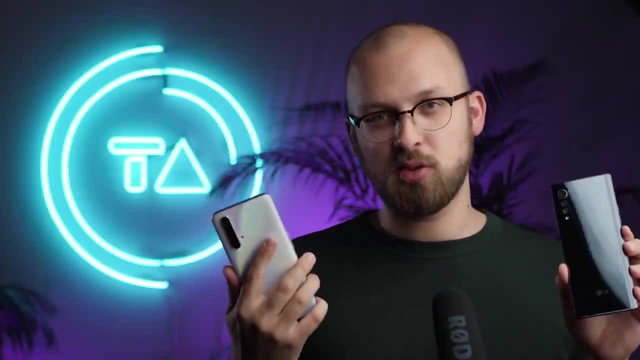 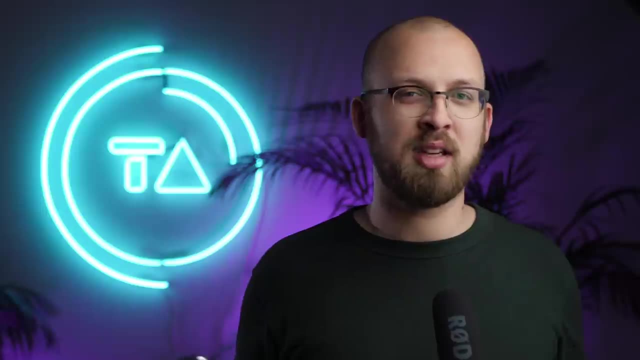 Now, the Velvet is the complete opposite of the X3 Superzoom, And that's because their target audience is the opposite of spec-hungry geeks, and their sales process is wildly different as well. The Velvet is sold almost exclusively offline. So the challenge LG had with this phone, 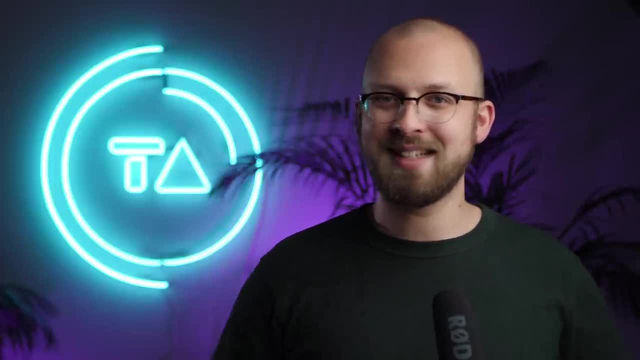 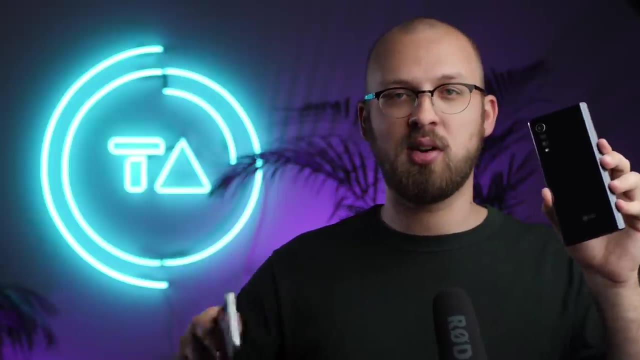 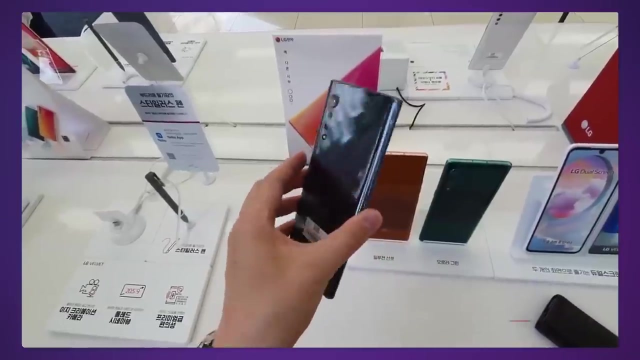 the thing they wanted to achieve was to create a phone that would convince a regular consumer walking into a physical store to pick this phone over all the other ones that are on display, And I think in that regard LG actually did a pretty fantastic job. So the LG sales process again starts with. 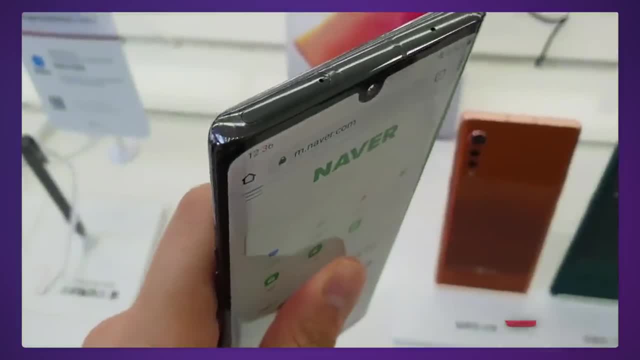 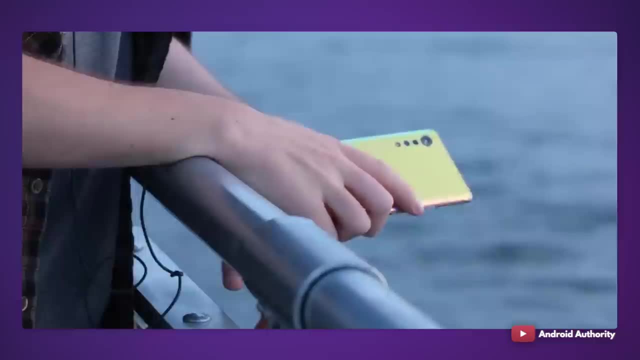 grabbing attention. Of course, in store, different things stand out to the customer, and LG's big accessories that are on display, as well as some of the insanely eye-catching colors, are designed to do just that. LG sent me the black version personally, for some reason. 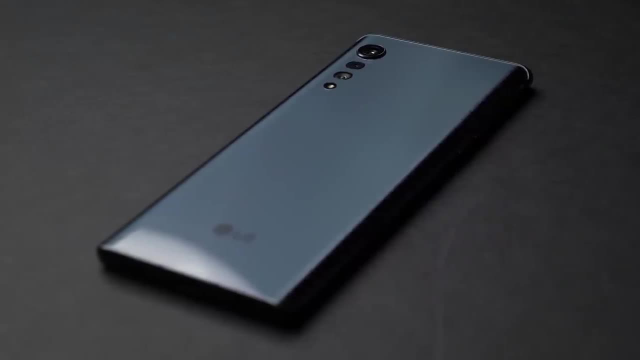 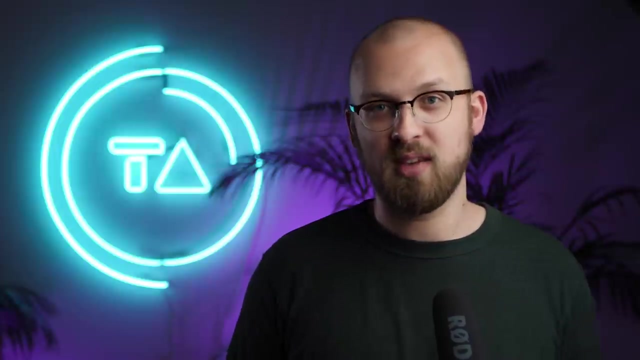 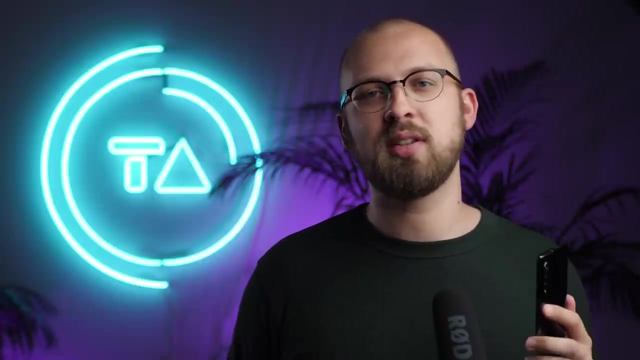 and that is sleek, but of course the least exciting color of the bunch. But yeah, that would surely stand out from the crowd on the busy store shelf. And then the consumer goes on to stage two, evaluation. And the things that we consider convincing as humans, in real life, in physical locations, are wildly different from the things 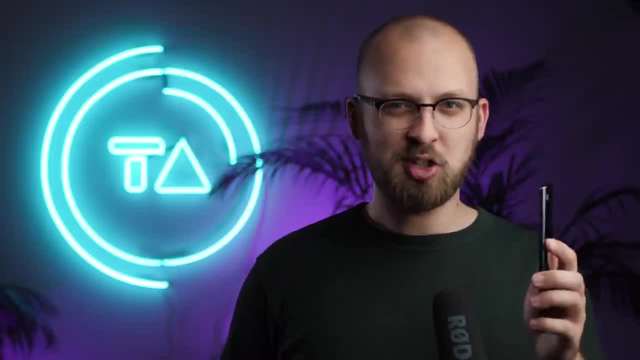 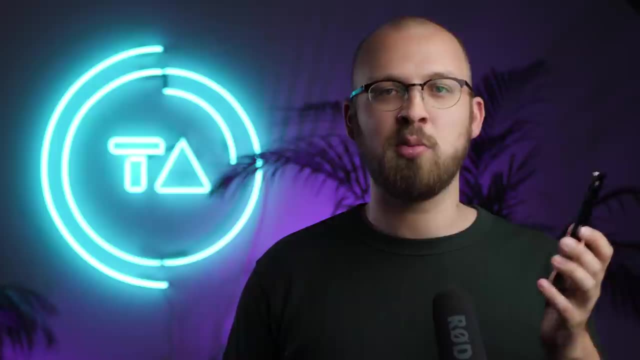 that we find convincing online. We touch these devices, we see them, we hear them, and our feelings, our visceral experience with them, is what overrides almost all of our other concerns, including those that we have, for I don't know the specs of a device. 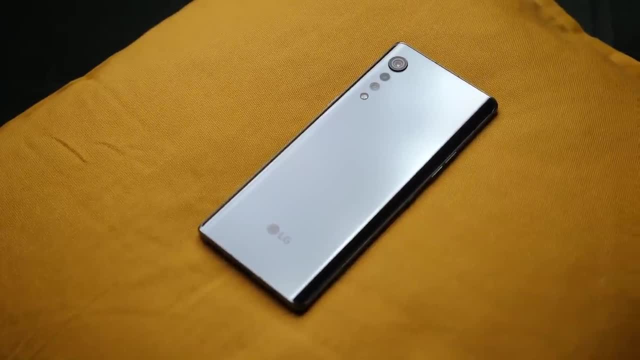 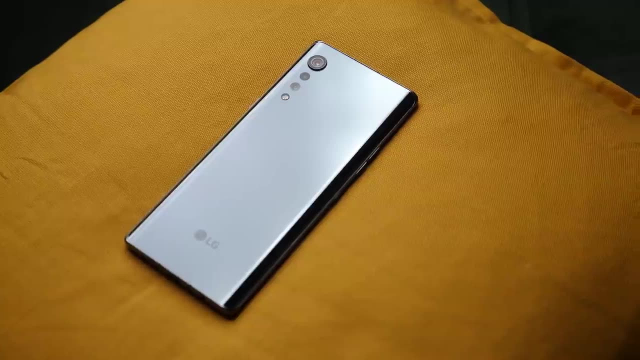 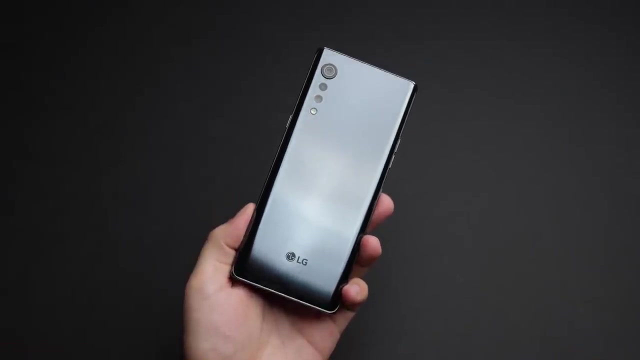 And I gotta hand it to LG. The Velvet in real life is by far the most polished device I've ever seen from them. It easily feels as luxurious and well put together as a thousand dollar iPhone or a Samsung flagship. It feels incredibly dense- all the corners, all the rounded edges. 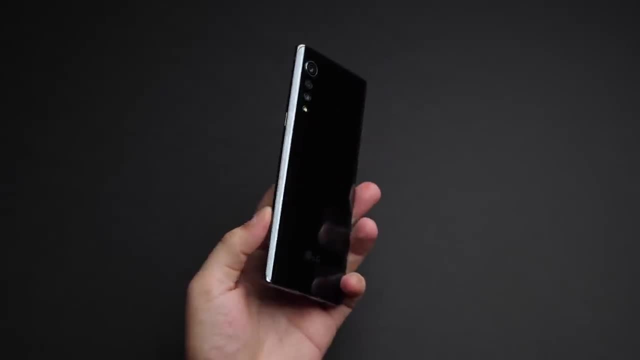 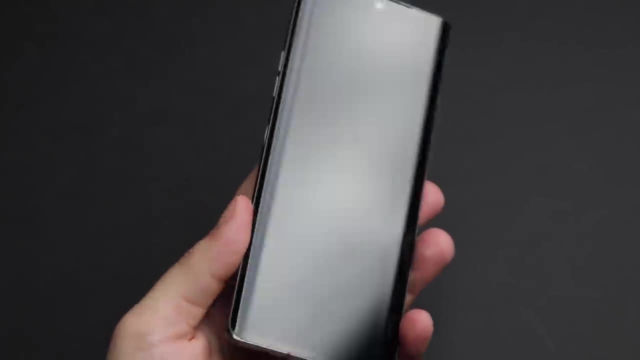 feel extremely well made. even if I personally dislike curved screens, The buttons feel great. the phone is 22 grams lighter than the real me, despite being physically bigger and glass and metal, and it is also thinner despite having a bigger battery, and that unmistakable. 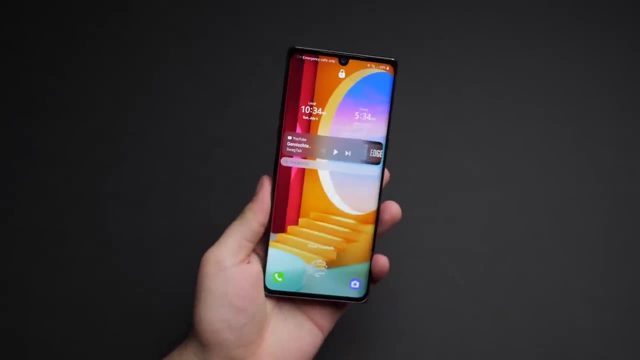 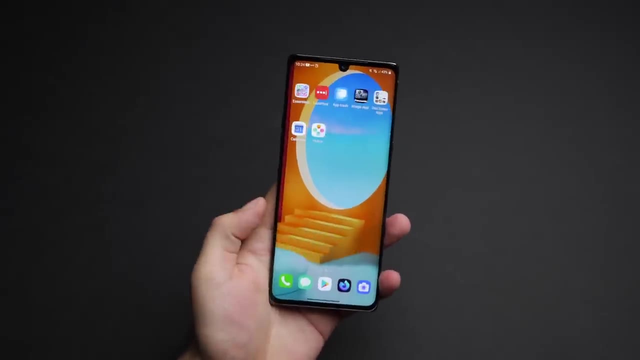 premium feel kind of carries through when you unlock the phone as well. This might not be a 120Hz screen, so it might not look as impressive on a spec sheet, but in reality I much prefer how it looks over the real me. In fact it looks every bit as good to me as the screen on my $1000 Note. 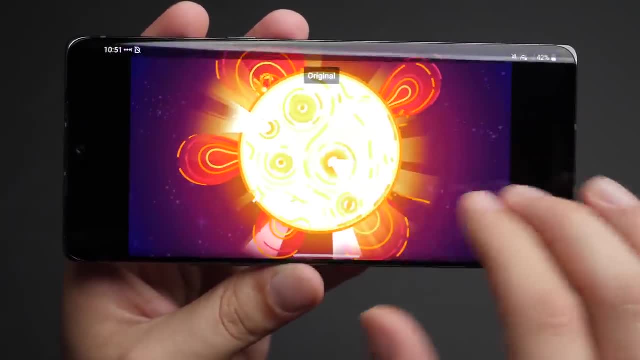 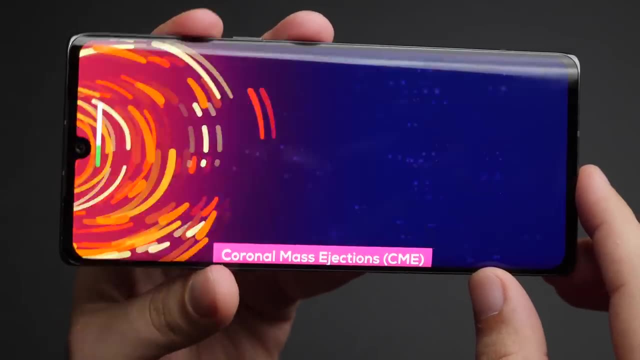 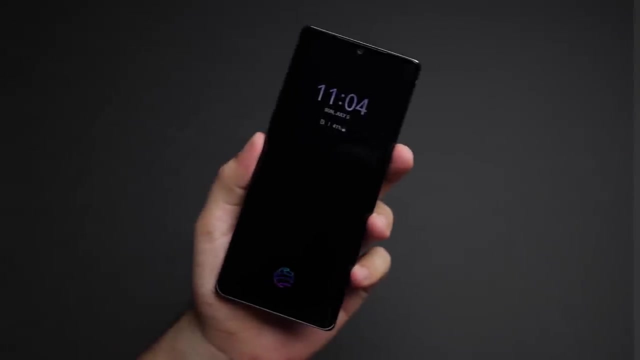 10, and all the other little things are great too. The haptic engine is solid and feels tight. the dual speakers sound way nicer than the single speaker of the real me, and I'm not sure people are ready to hear this, but I even think the software looks attractive on first glance. Obviously, this is 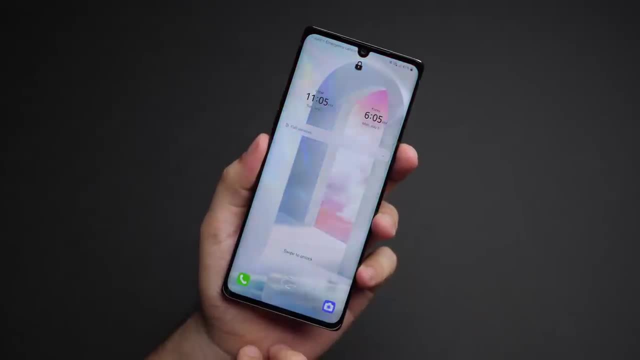 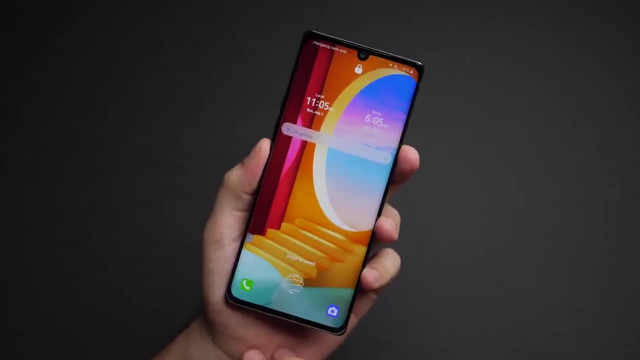 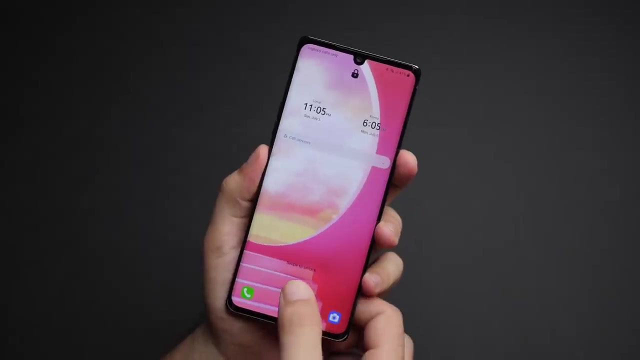 even more subjective than everything else I'm saying, but I think everything from the always on display to these animated lock screens that keep cycling through beautiful custom wallpapers, I think these are the kind of things that make the target audience go into a shop, try it out and go. 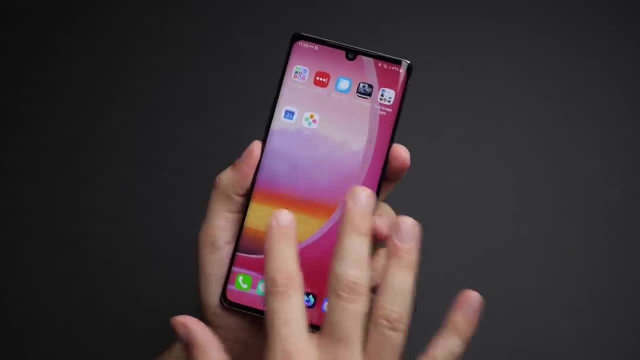 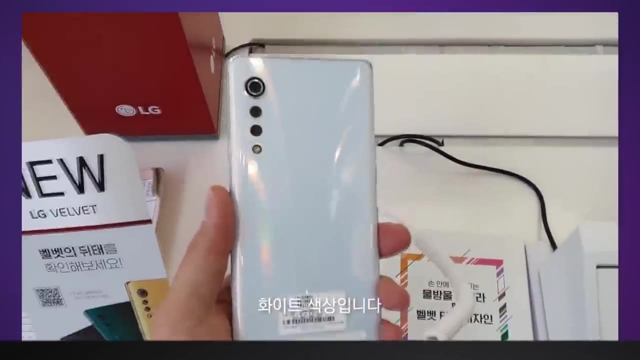 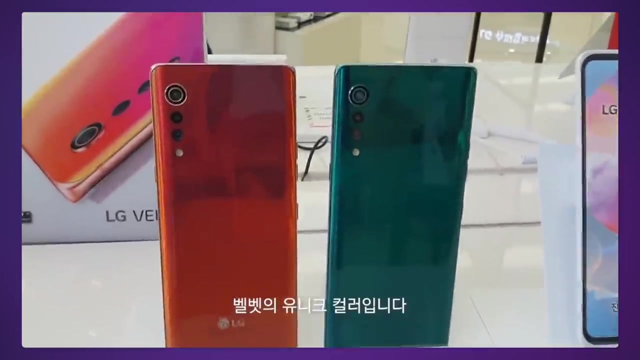 pretty. I want that, And that feeling of instant in-person desire is what LG has clearly spent a lot of time and money on. For this sales process to work, the customer has to pick up the Velvet from a busy store shop with many other devices, and then they have to fall in love with it from the first. 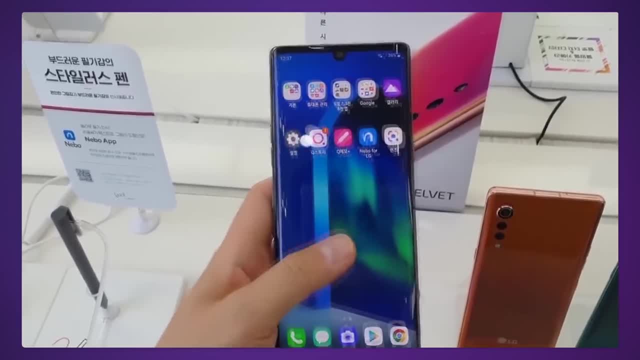 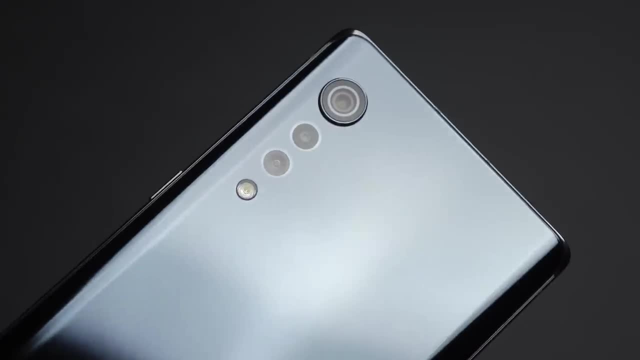 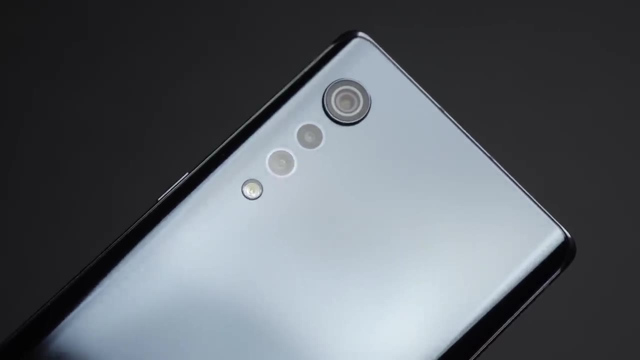 touch The first click of a button, the first lock screen animation, the first buzz of the haptic engine. those are the things that matter, And everything else from the slightly slower processor to the air quotes. only 6 gigs of RAM. well, those are corners LG had to cut to maximize this feeling. 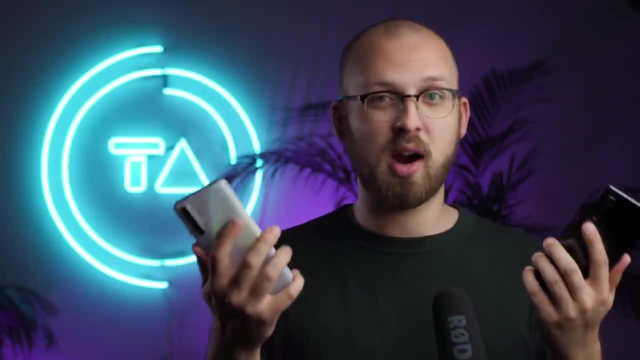 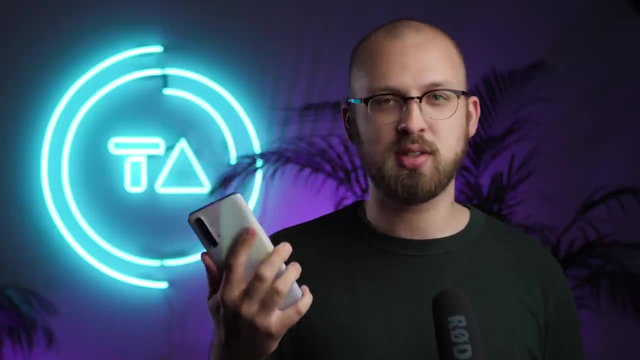 These two phones are so wildly different because they're made for wildly different purchasing processes and I've always felt like real me, really understood their process and made all the right choices for their specific process and for the specific target audience. but I feel like with LG. 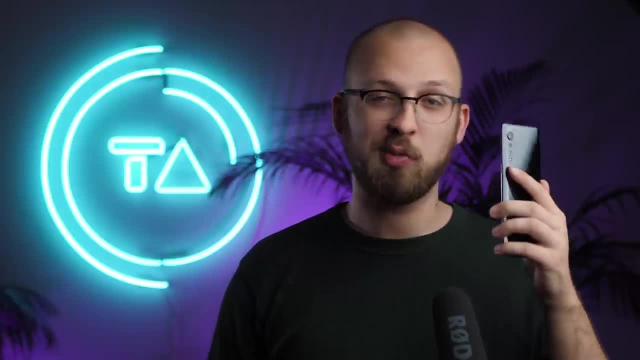 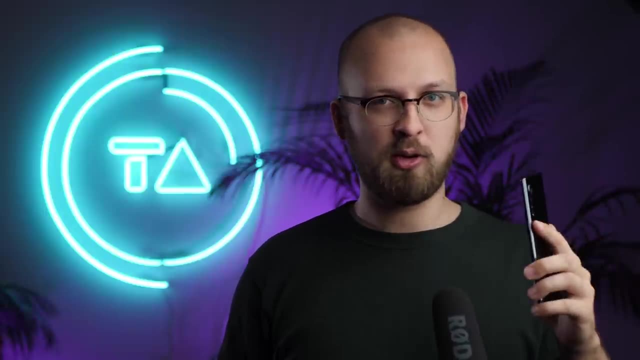 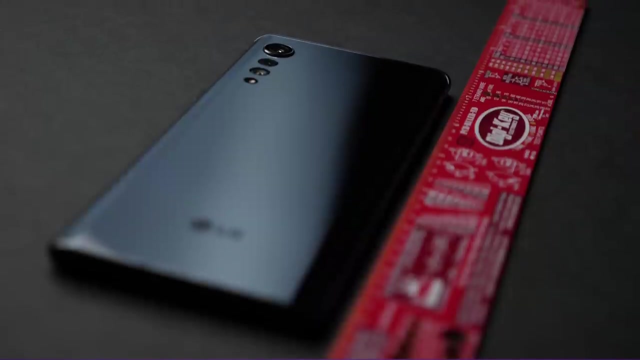 the Velvet is their first phone in years where I feel like they really nailed it. It might not be the people who watch my kind of videos, but I think for a phone that is supposed to sell offline to regular people, this is a killer device. Product design is both an art and a science.